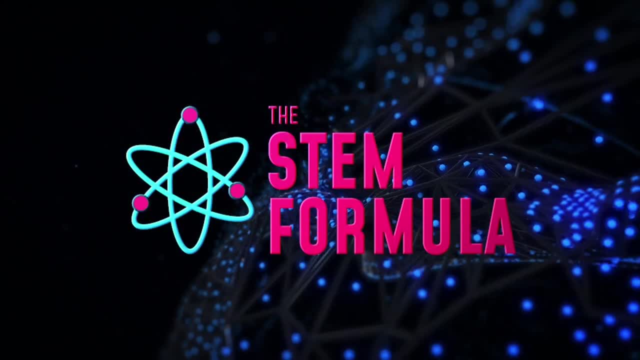 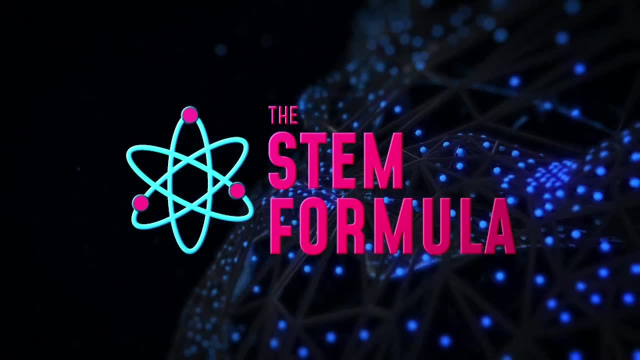 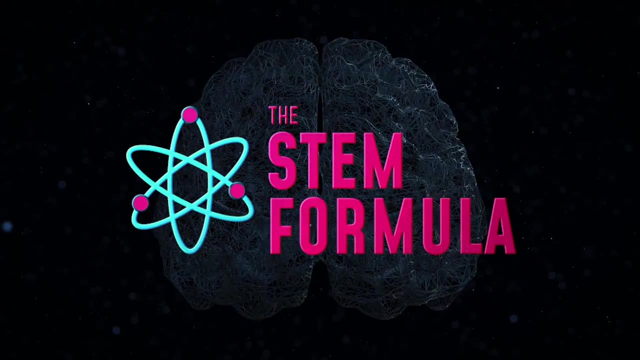 Welcome to the STEM Formula, a podcast from the residential campus of the Governor's School for Science and Mathematics, located in beautiful Hartsville, South Carolina. In this podcast series, we enjoy a down-to-earth, straightforward discussion about advanced STEM education. Hi, I'm Michael And I'm Nicole. 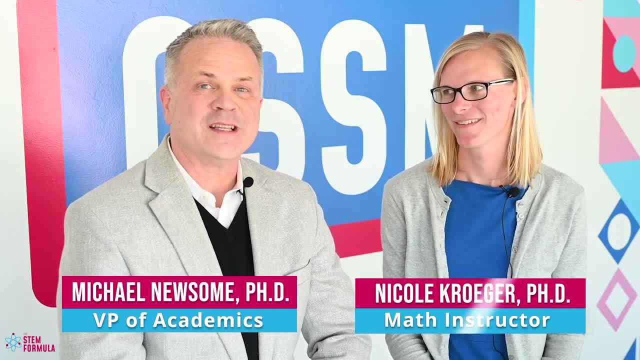 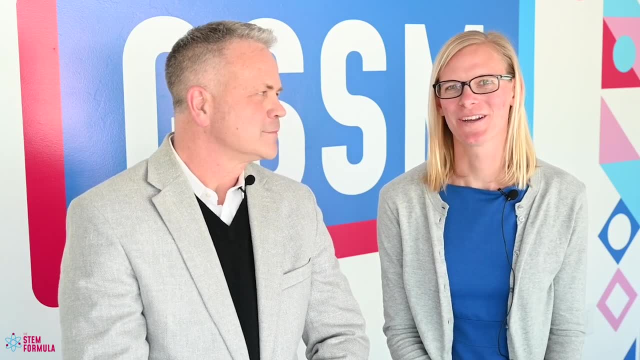 Nicole, it's good to have you back. While you were gone, we were able to interview Dean Cynthia Young at Clemson and architect Alex Lay in Greenville. So who do we have today? We're talking to Dr Kristen Walker, a physics teacher from the Governor's School of Science and Mathematics. 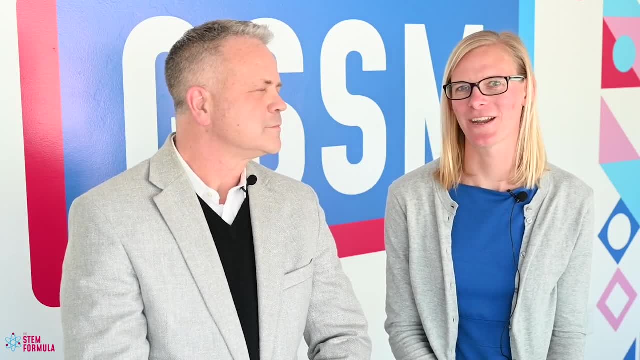 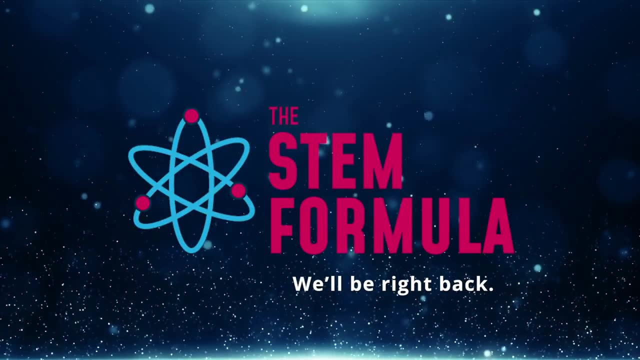 She has extensive experience teaching physics with us and has great advice to share with us today. Yeah, Dr Walker is also one of our department chairs. Hi, Kristen, Welcome to the STEM Formula. Thanks for joining us today. Thank you, It's good to be here. 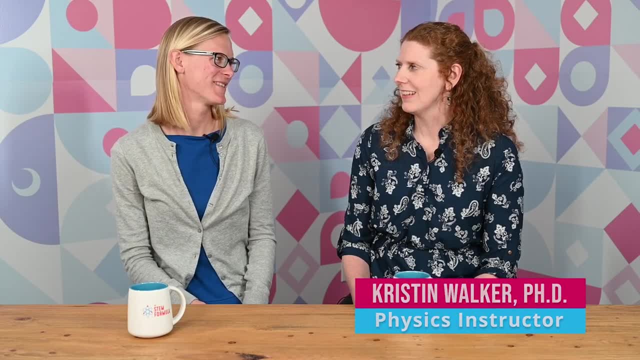 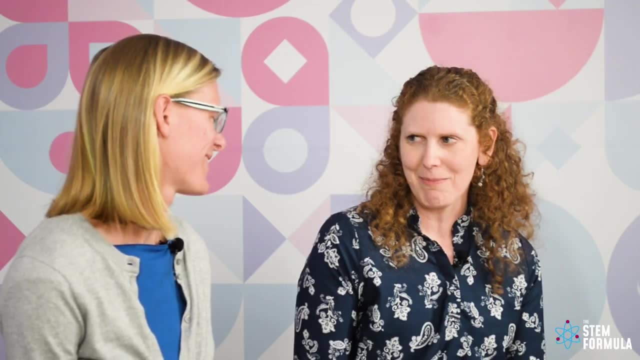 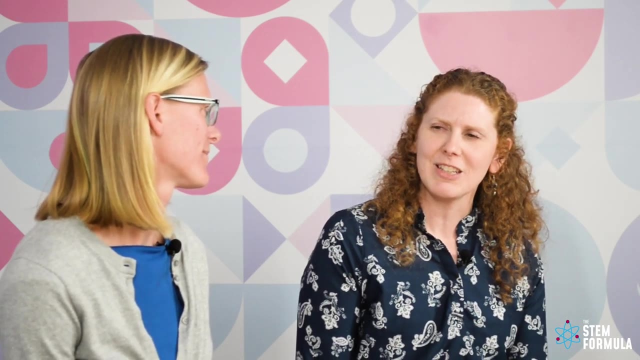 Can you start out by telling us about your background and how you came to the Governor's School? Yes, I've always been interested in math and science, especially math, And Got into physics because it's applied math Throughout. my undergrad realized that I enjoyed teaching, but I wasn't sure what level I wanted to teach. 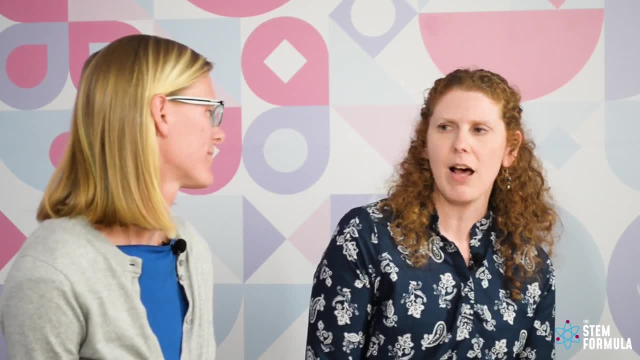 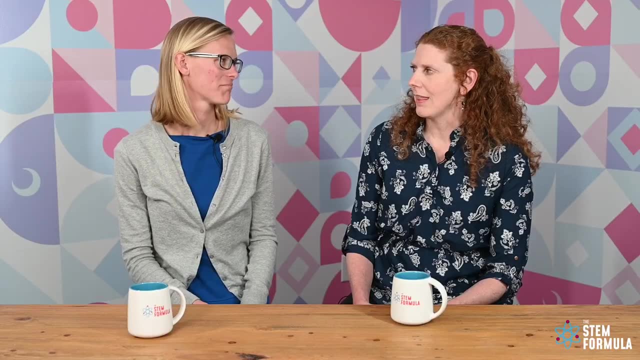 Didn't really want to teach high school. So I went and got my PhD in optical science and engineering, working with controls, correction systems for telescopes, And then through that, through my TA, and I realized how much I actually enjoyed the education side. 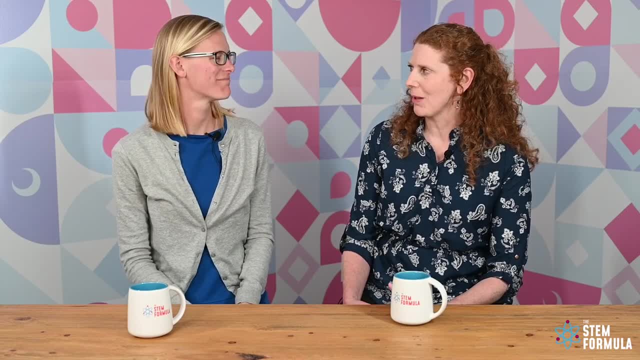 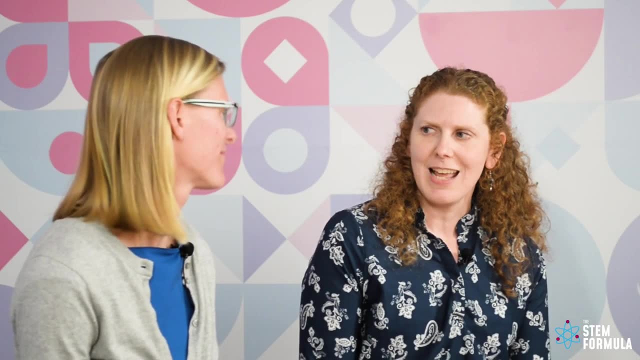 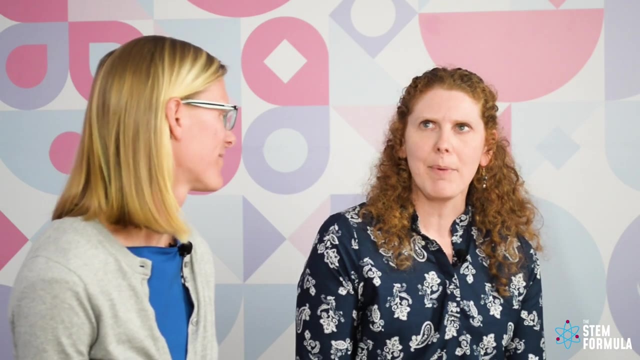 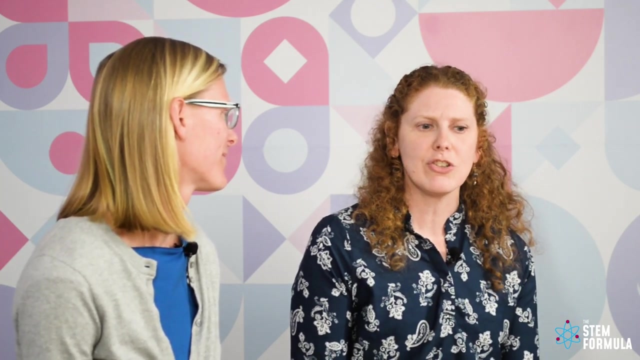 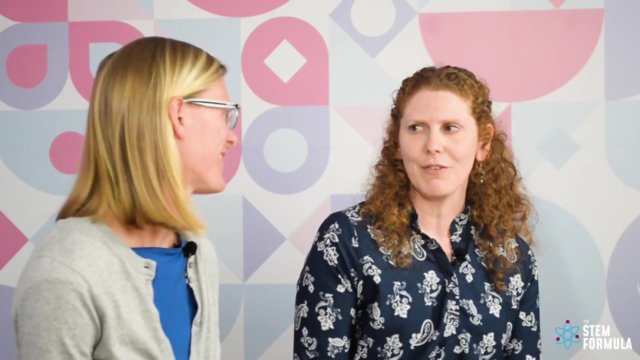 And actually my graduate school was more for the education. I was a black sheep in that regard of not wanting to do that, Taught at a small liberal arts college for about five years And then this opportunity came to teach here. I was a little hesitant to come to the high school level after teaching college, but I realized the opportunity to impact students at a younger age, when they're still figuring out what they want to study, still trying to figure out what's out there in terms of the STEM field- that I really appreciated that here at the Governor's School of reaching them at a younger age. 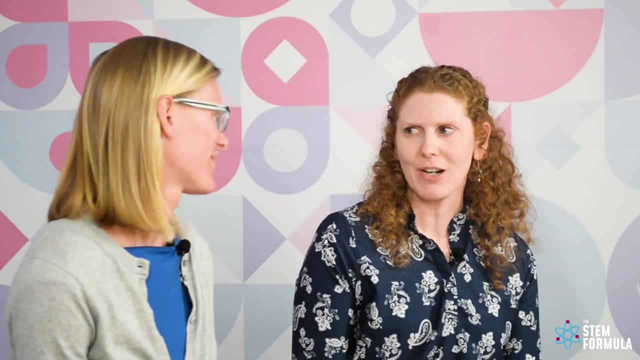 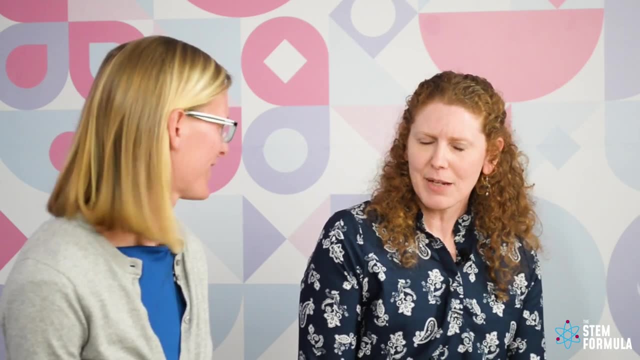 And not later, when they're already set in their college career. But that's so. that's why I come in here and I'm enjoying that. I'm enjoying that chance to let them know what physics is the first time they're seeing it, and then they still have some opportunities to decide their field of interest. 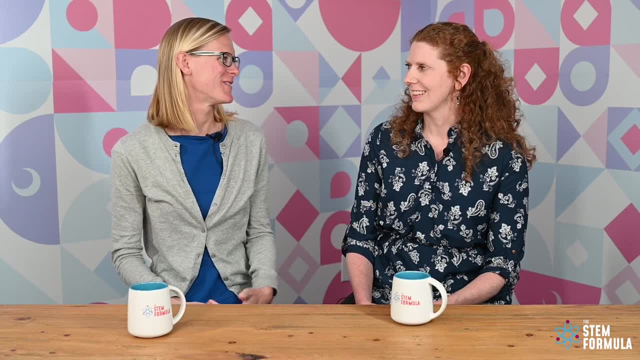 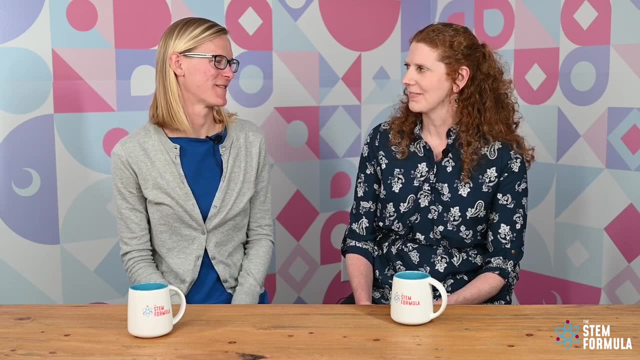 Yeah, that's a lot of fun, And one of the ways you get to impact students in a way that you might not at a college is you've been teaching some interesting elective classes- physics and the arts- and you're adding a physics in the sport or physics and sports class soon, right, 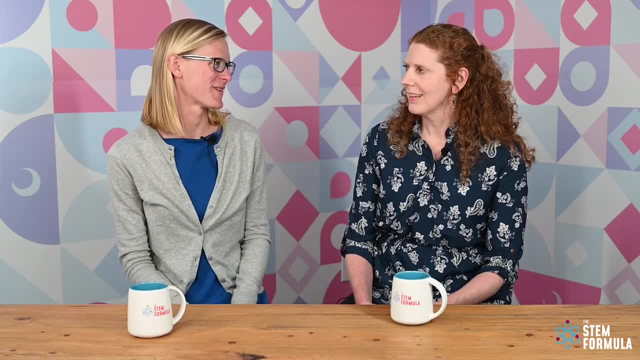 Can you tell us a little bit about those classes And how you reach students in those particular classes? Yeah, because we have we one of the things that the Governor's School is. all the students had to take physics somewhere in their career. 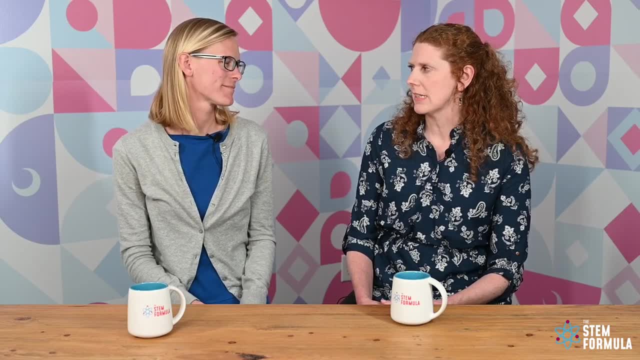 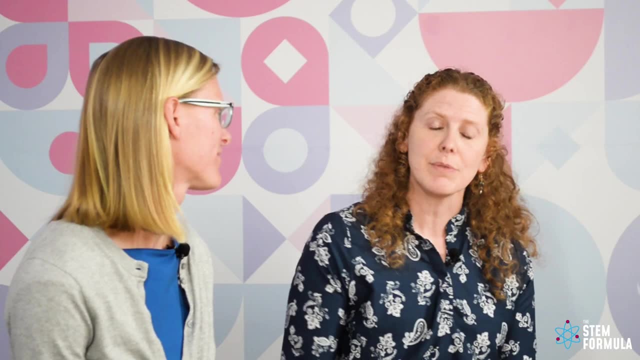 So we cover the basics of mechanics, electricity, magnetism, but, like I said, there's still high school students and they may not take another physics class, especially if they have some dual enrollment. So I enjoy optics, I enjoy arts and music. 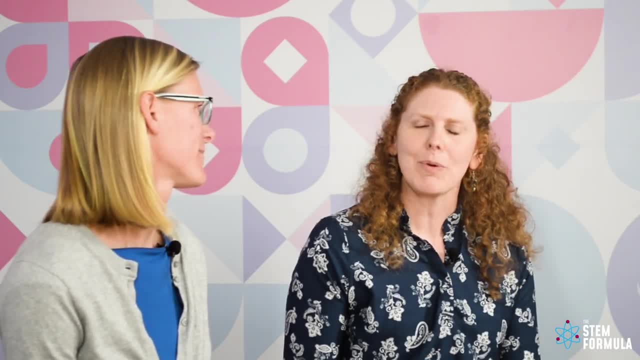 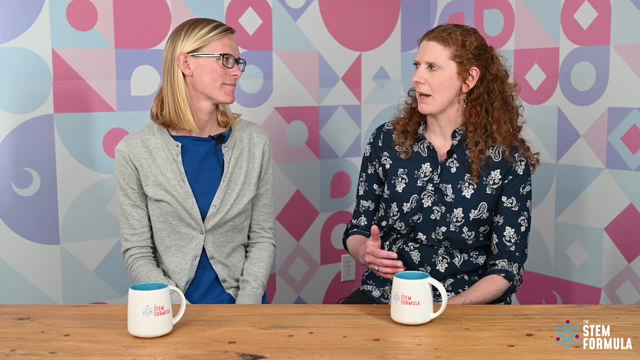 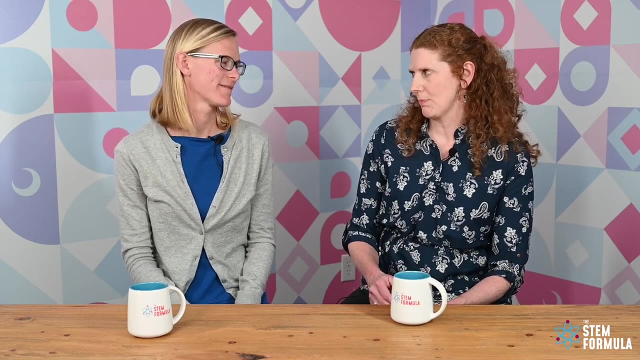 I play musical instruments and sing, So I wanted to incorporate that in the curriculum. So I came up with this physics And the arts class that's meant for students still have to have the same math experience as a normal physics course, but they don't need to have had the full year of physics before before taking this course. 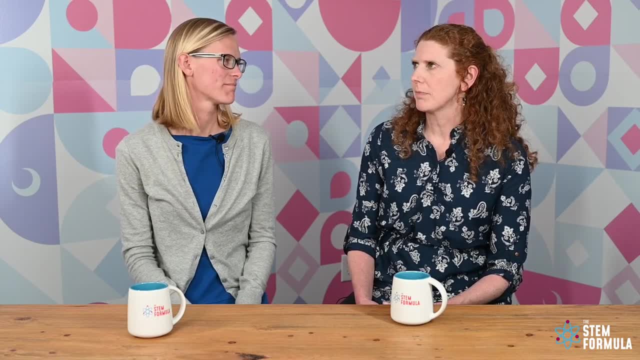 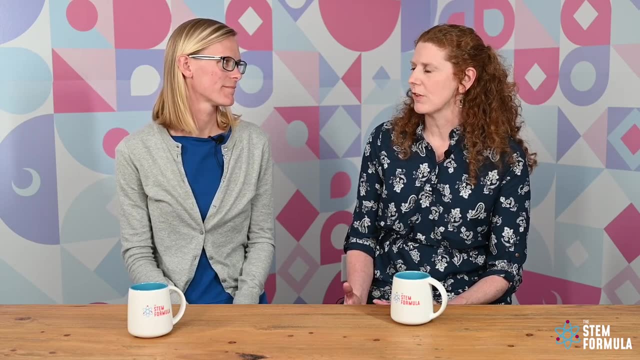 So we do half of it with music. We talk about musical instruments, musical scales, talking about how different mouthpieces like a trumpet versus a clarinet reed work, and going into some of the details with that. So that's half the class. 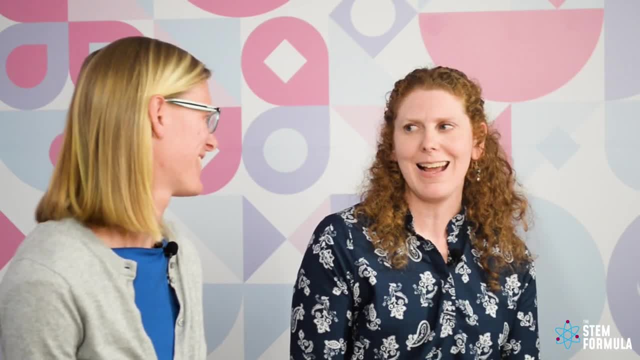 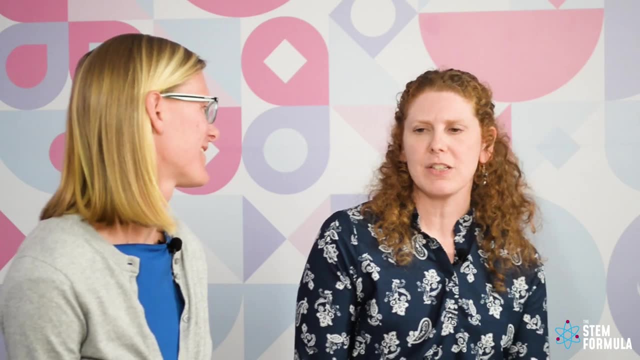 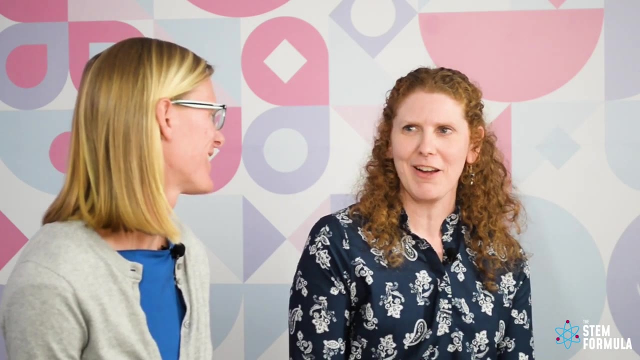 The other half is looking at Photography and looking at the optics. That's where I can really bring in my PhD Love into that. And then we also go beyond the normal physics curriculum and going into some color mixing, talking about history- as she we always do class where we talk about history of record players and photographs and going into cassette players for the music side. 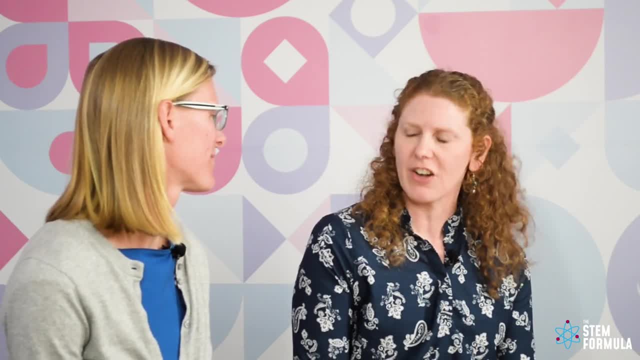 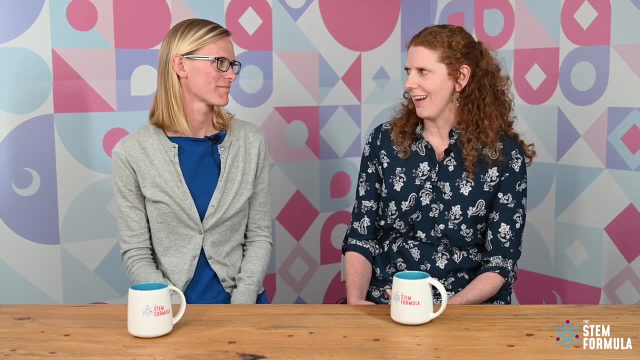 And we also do some of the history when we're looking at the photography side. It's also a fun course because I can be a little bit more interdisciplinary And bringing in the biology of the eye, the biology of the ear. so I've been doing that. 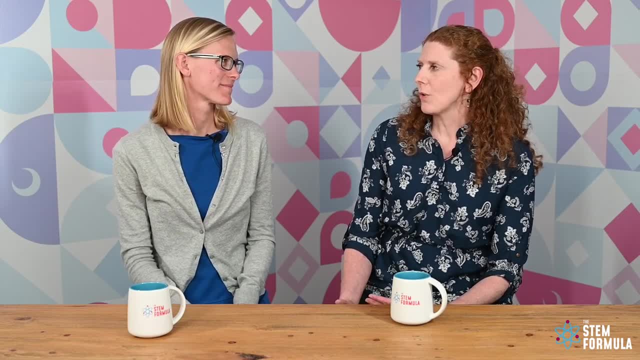 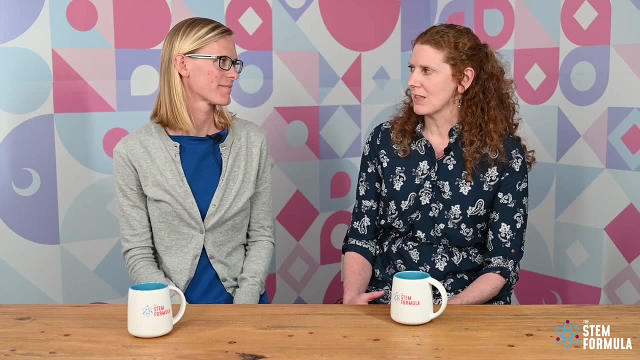 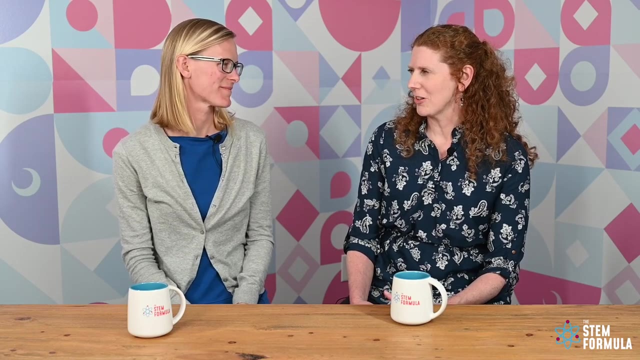 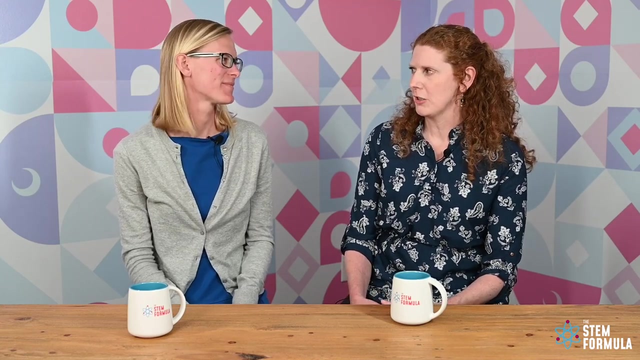 So I'm proposing introducing a new course next year. physics of sports is. a lot of our students are interested in exercise science- My previous job- there was an exercise science kinesiology class, so I might bring in some elements of that. so I'm going to talk with some of my biology colleagues and brush up on some anatomy physiology, but bringing the visits of the body, the kinesiology part, but also looking at 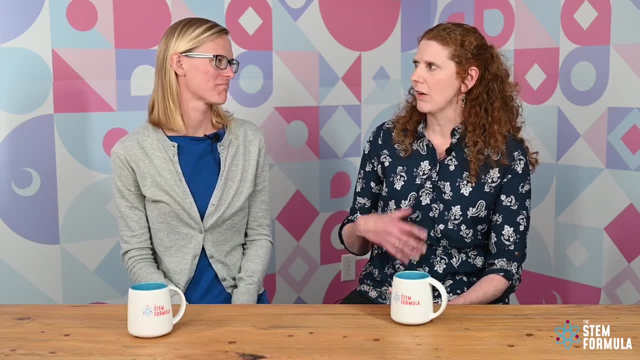 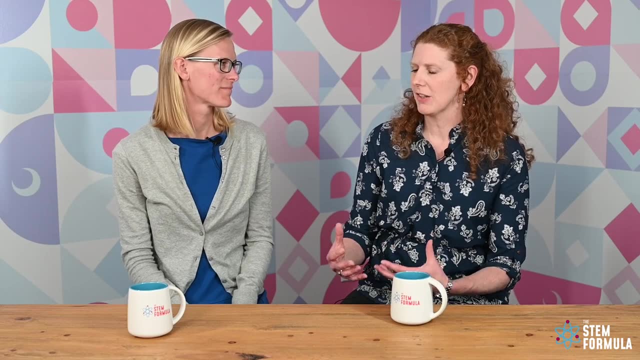 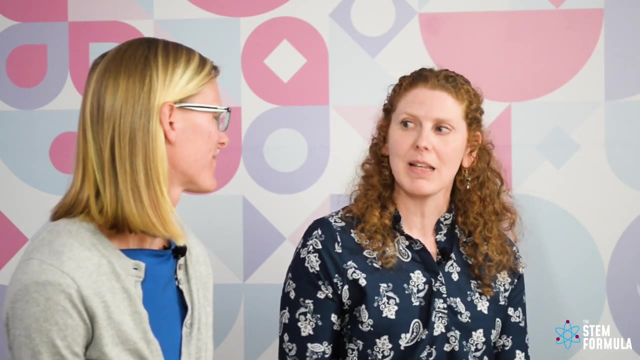 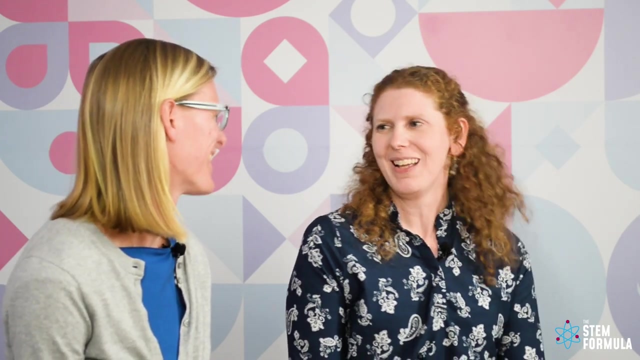 Some of the physics of athletic equipment. why do curveballs curve? looking at golf club angles, looking at rackets and the body. so looking at the physics of the equipment and also the physics of the human body, depending on the interest of the students. and same thing, trying to make it interdisciplinary, bringing in some interactive labs to help with that as well- go to the, go to the gym- and trying to figure out different muscle groups in terms of the exercise. 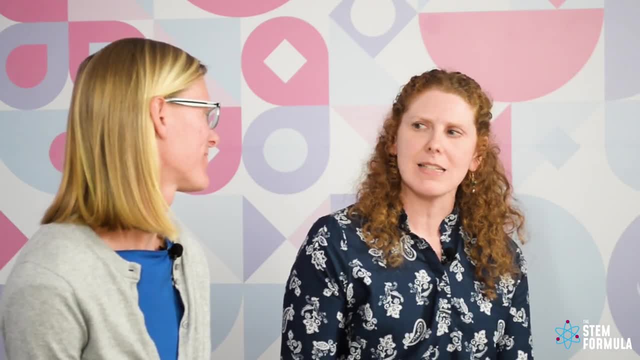 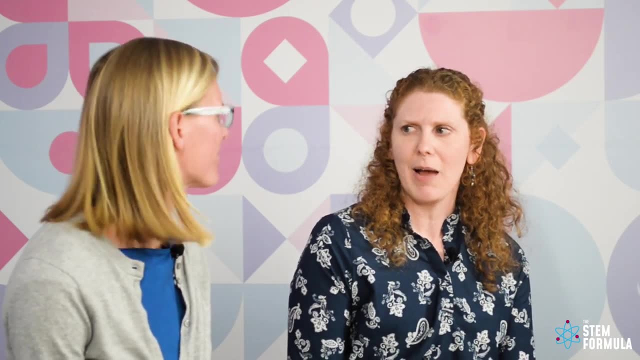 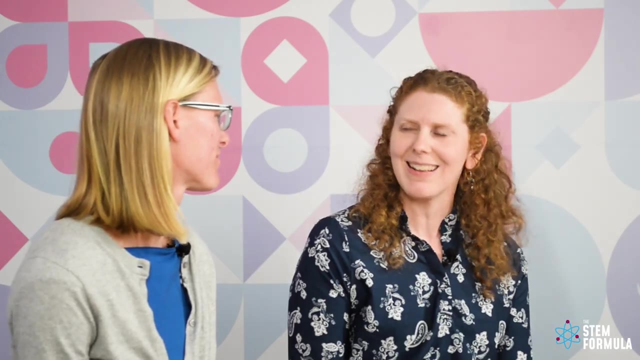 So that way, My, My goal, especially for that class, is the students, especially biology students that have to take physics but maybe want to learn a little bit more of the biology applications going into exercise science. So that's some of the outcomes, hopefully, of that class. 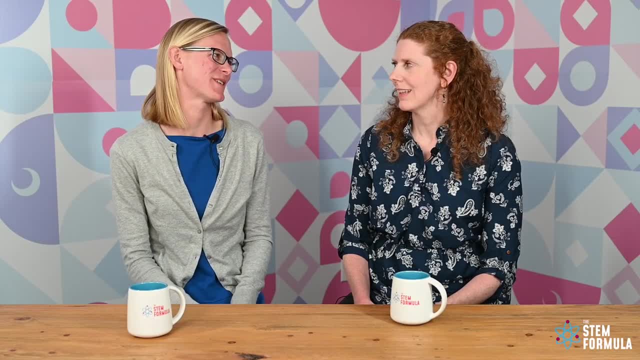 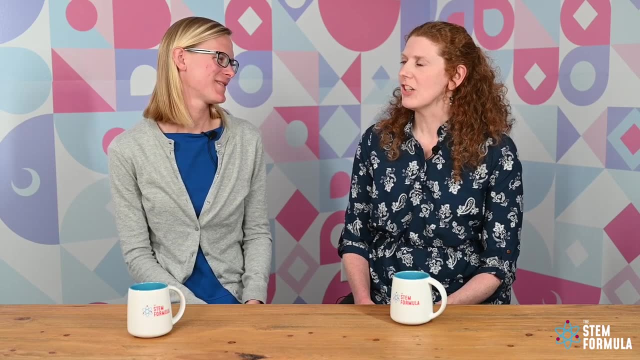 So, Kristen, both of those classes sound really interesting. Can you think of a particular like unit or activity that you do in in those classes that could be used by other teachers? Yeah, actually, the physics of sports was inspired by my internship. 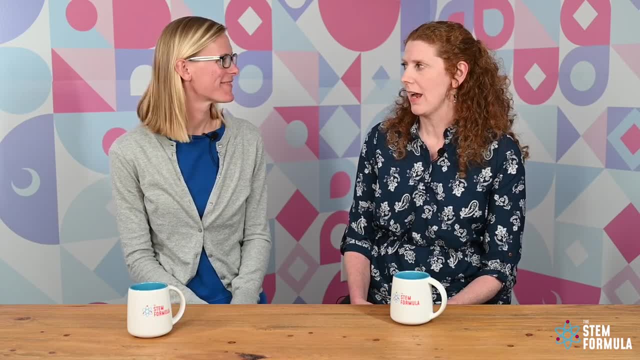 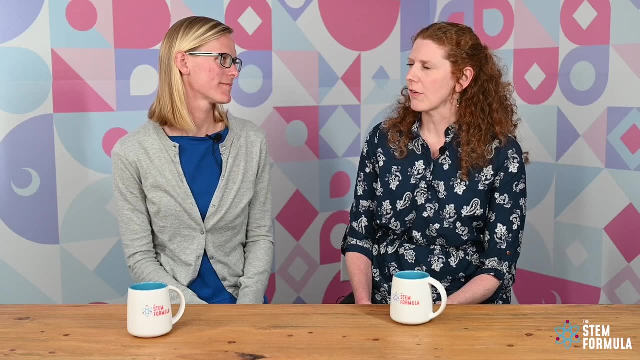 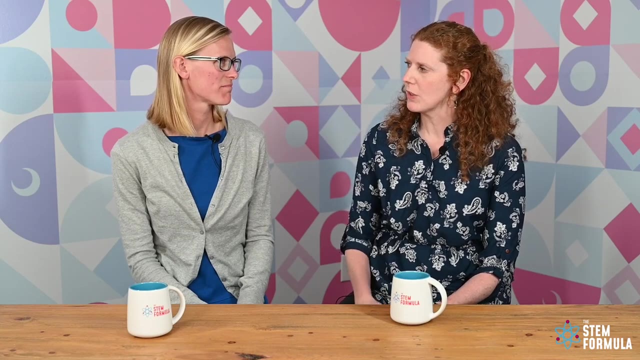 I took an interim class, I helped with a colleague where we did sports and I took a couple of classes, just one hour sections talking about sports. So even just looking at center of gravity, of looking at the human body, of this idea of when you're high jumping, you actually have your center of gravity below. 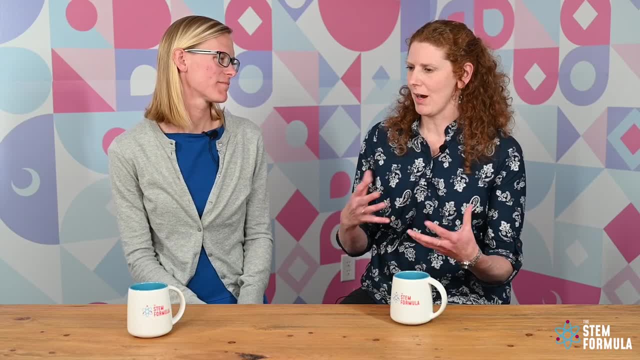 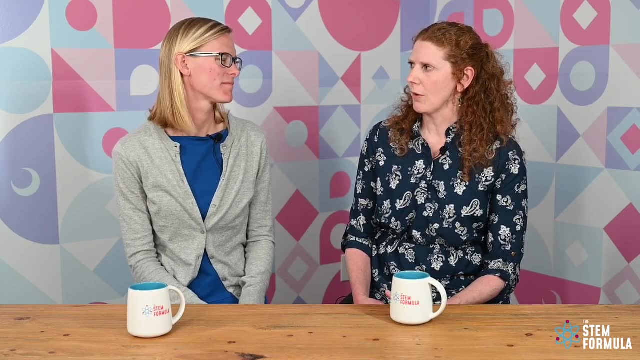 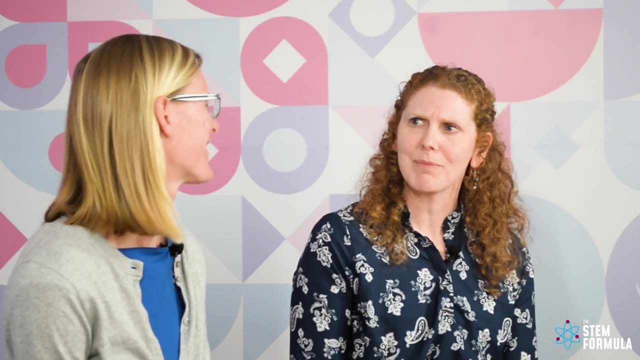 So there's a lot of activities for physics or biology: looking at center of mass and looking at just the normal, your body moving back and forth- that can be helpful. and also looking at high jumps- So I would probably be one little unit- and also looking at the curvature of balls, putting a top spin, putting a back spin on it. 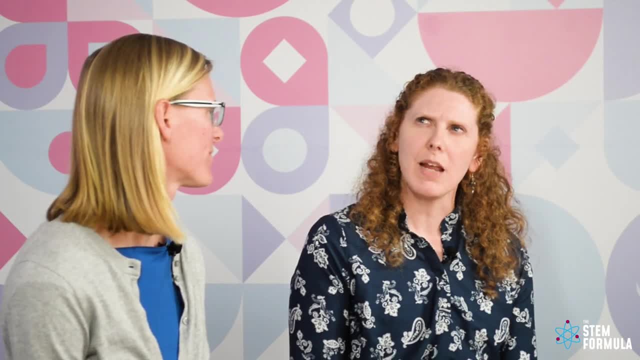 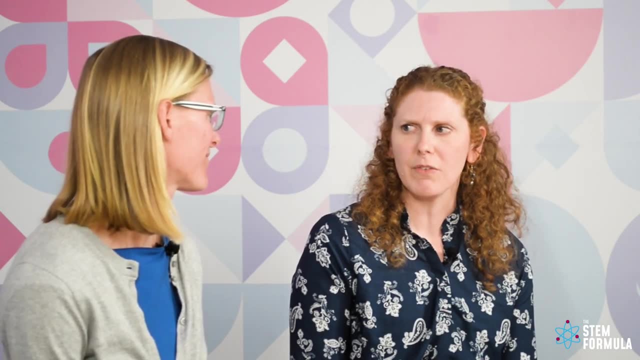 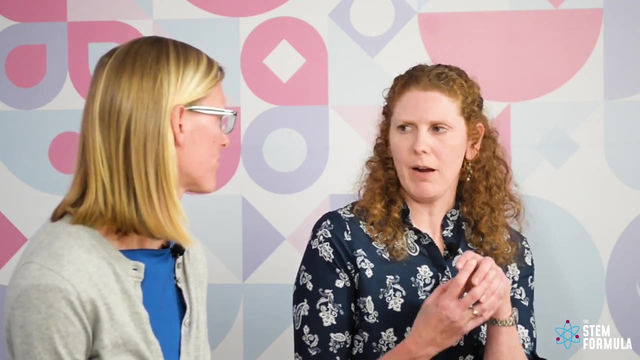 So even that in itself could be a short unit, I would say within the optics. just looking at photography, that's a very easy way of how does a camera work. looking at the optics involved getting some laser pointers and even just common. even if you took a bottle of water, that works as a lens itself. 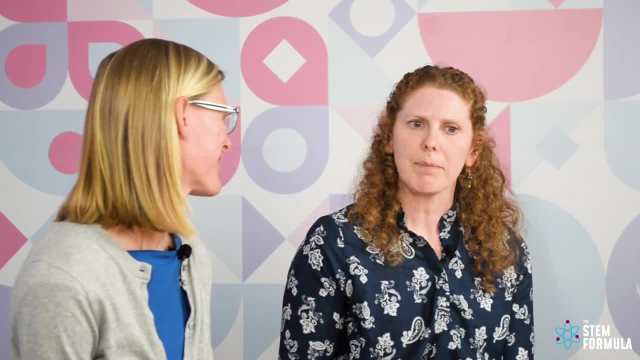 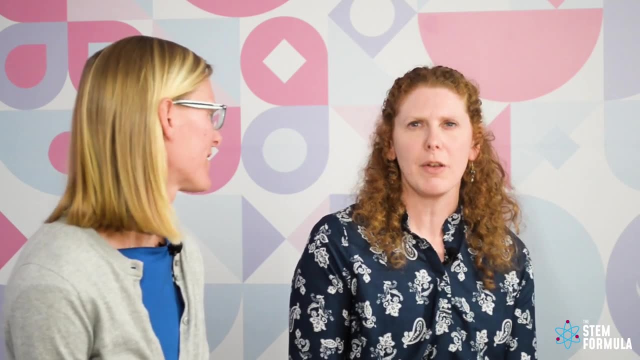 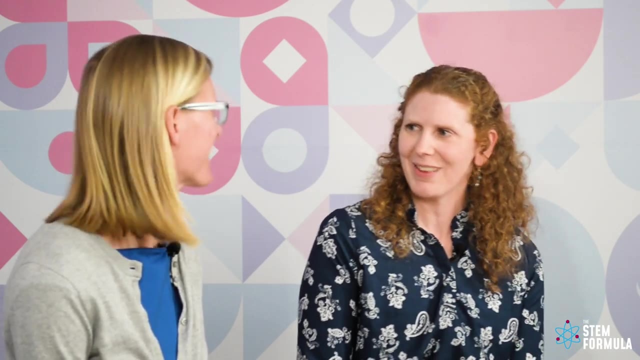 So there's some other Ways of bringing in the bending of light for the photography part of it that can be a self-standing, along with color mixing. So some of that's already currently taught at different levels in the physics, but those are ones I bring in all together within the physics and the arts and physics of sports classes. 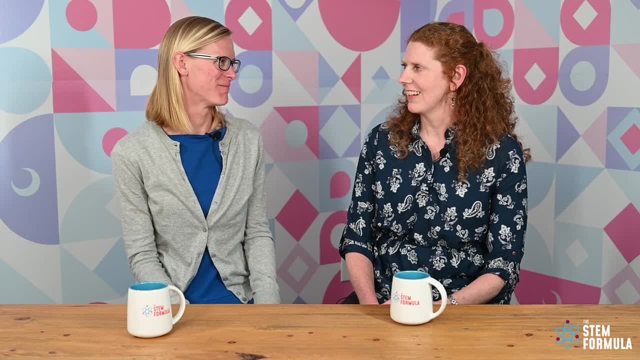 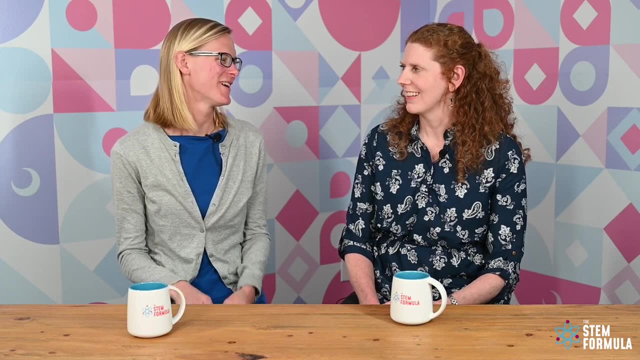 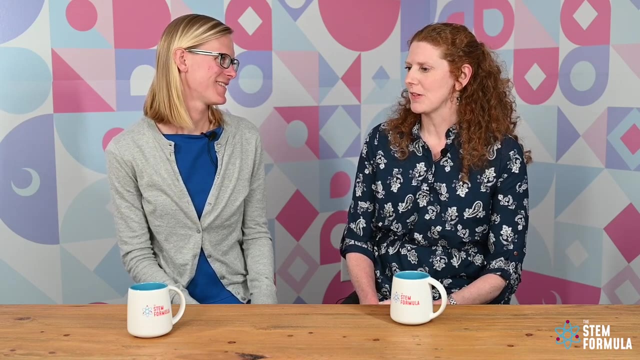 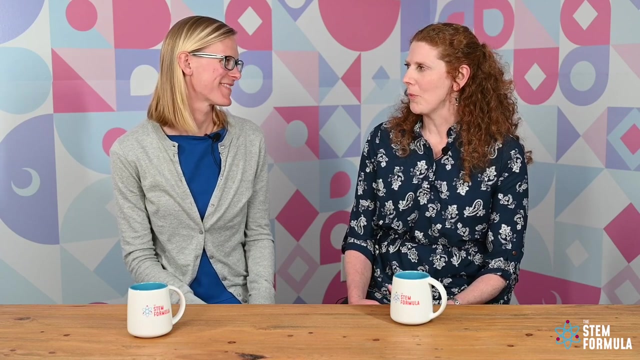 Awesome. Those are great because there's some, like things that can be done with ordinary objects or things that you already have available. So that's really awesome. Are there any demos that you do in your, Like, general physics class that really stand out as something that you would like to share with our audience? and we have? you know, there's all sorts of demos you could get with normal physics equipment, but some, um, we are currently doing we did waves and sound and I do a whole one man bandstand in class one day. 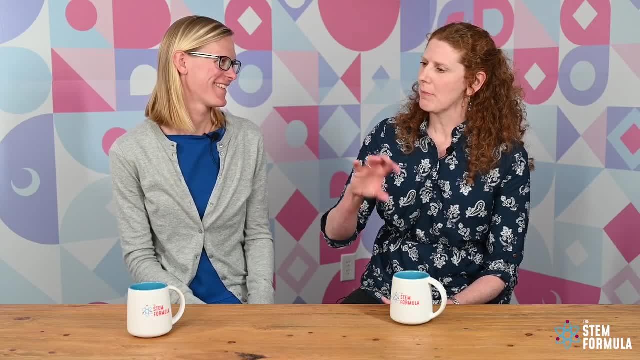 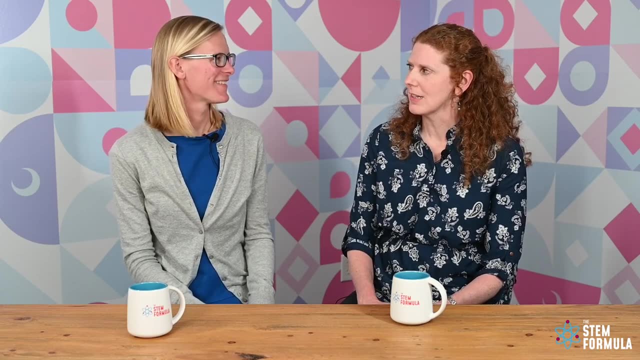 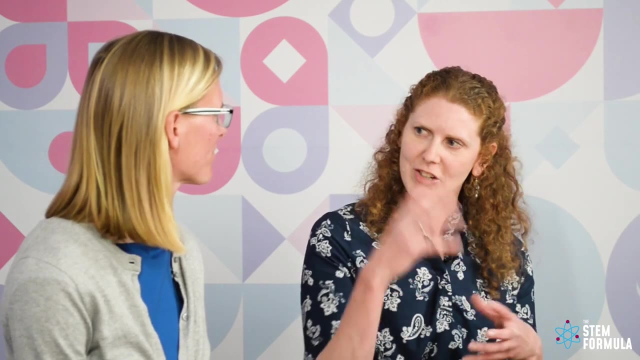 So, taking wine glasses, playing the wine glasses, seeing what happens when you add water, what happens to the pitch. same thing with glass soda bottles of what happens when you hit it versus blowing across it. There's some everyday equipment, Um so resonance. you can take a hair scratcher, a hair massager, and when you pluck one of the tongues, the long ones vibrate but the short ones don't, and vice versa. 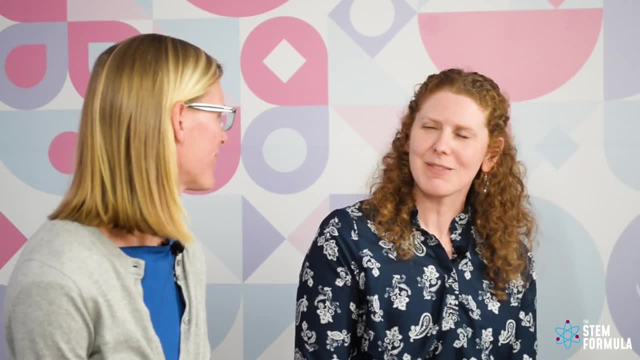 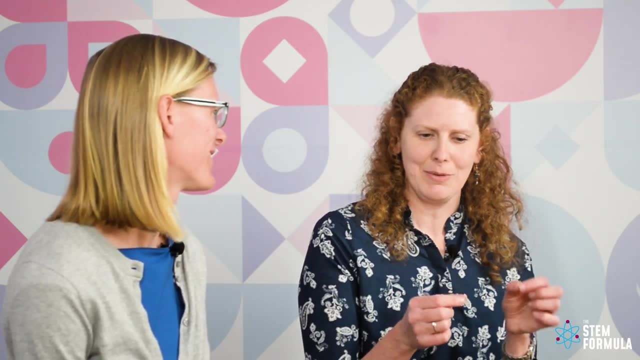 So there's little things like that. I'm actually going to talk about fuses. We're talking about electricity right now, And if you take a copper scrub pad and you take a little piece of it and connect it to a battery, it does go and get very hot. 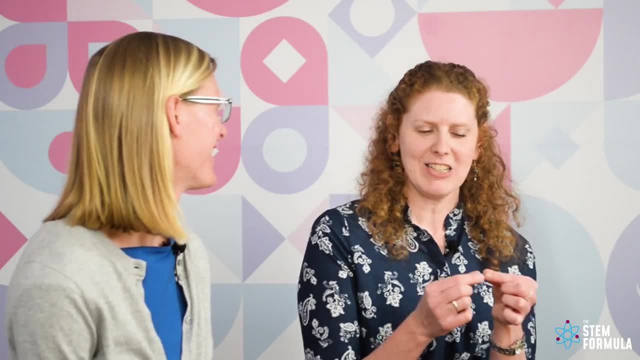 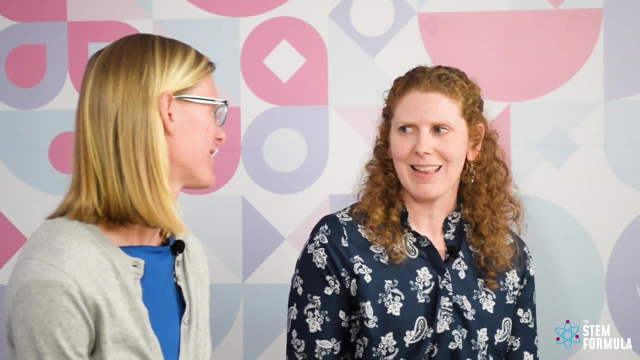 So super. I can't tell this at home, but there's a sense that you can actually see how the fuse gets hot enough to break. and talking about how a fuse and breakers work, Um, because a big thing with physics is trying to bring in the, the real world applications. 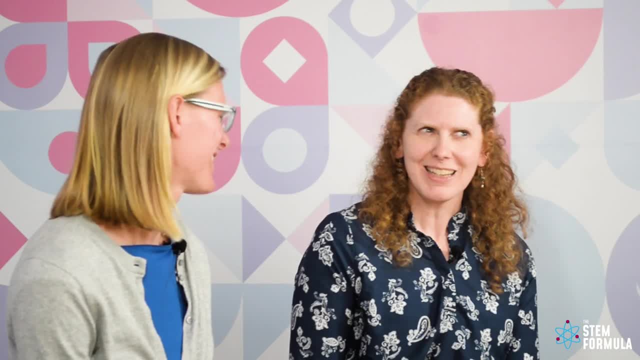 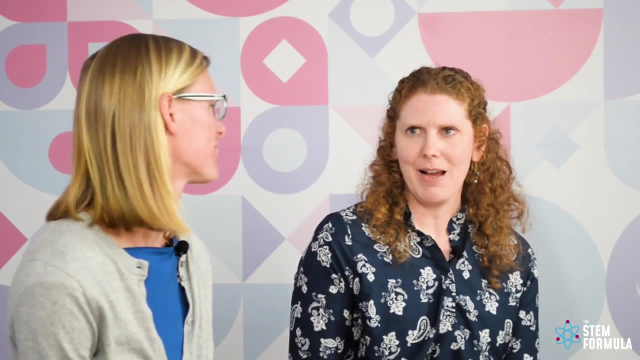 It gets very math heavy And, as you know, the math, why do we need the trade? Why do we need the math part of it? But there's a sense of trying to always relate it back to everyday items. Um, so those are some of the demos that we do, that I do. 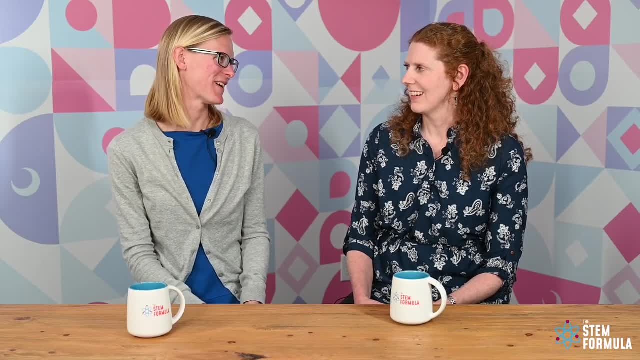 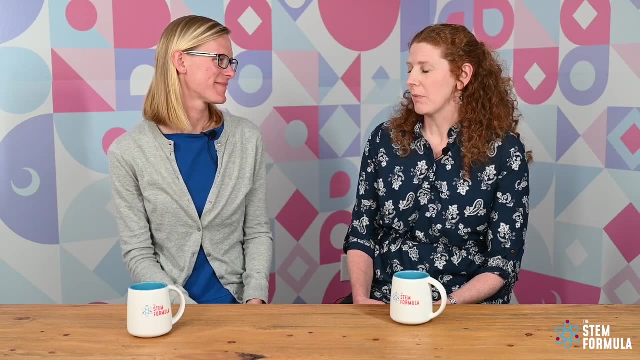 And can you do you have any last minute advice for teachers out there? I would say that definitely the big thing with with physics, as with any science, but it's especially physics because it's everywhere- Is always relating it back to real life things. 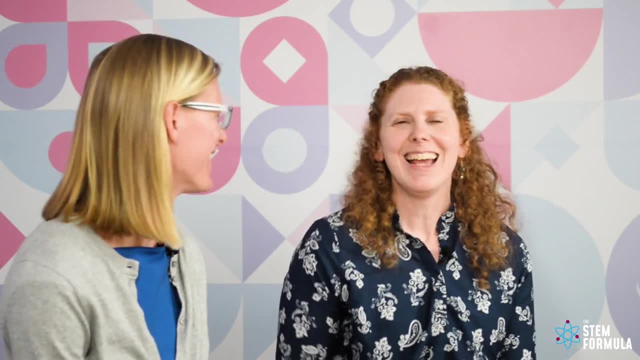 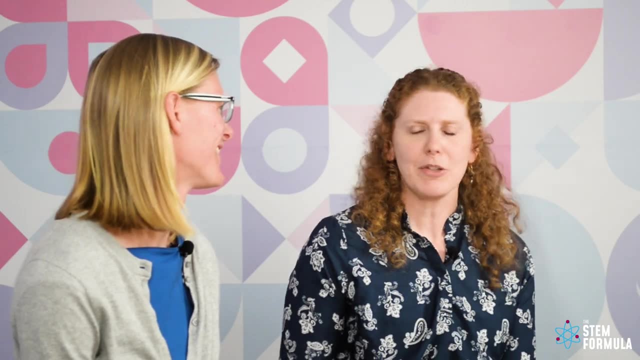 How about when you're trying to change a tire? What type of equipment do you need um changing a battery? How did the circuitry work with that Um? and also, just even though they're young and I showed them a breaker box the other day- they may or may not know what a breaker box is at the high school level, but always bring it back. 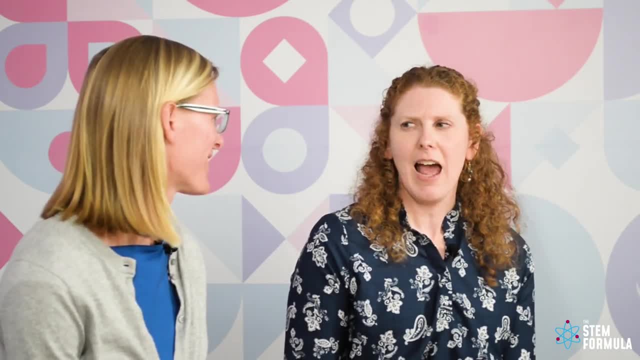 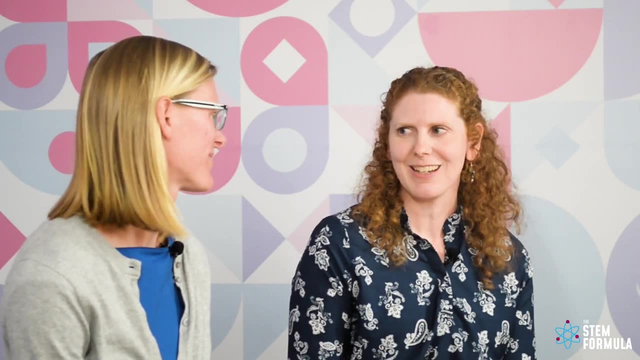 So that in those stages when they do see physics they have that connection. So really just trying to always bring it back to application. Same thing With the, the sports, with the arts, the music, um, bringing in the application part of it. 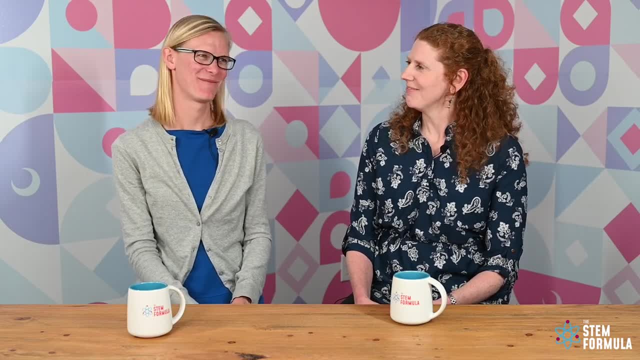 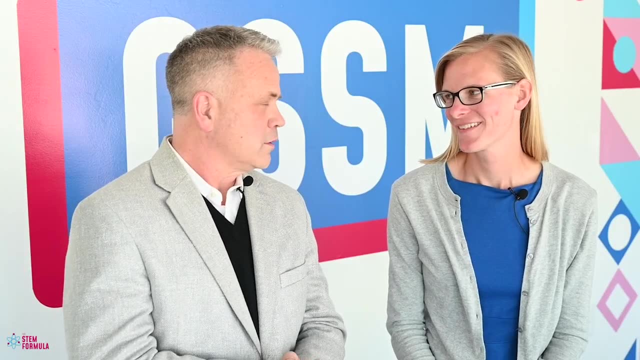 Wonderful. Thank you so much for joining us today, Kristin. Thank you Now, Nicole. you've known Dr Walker for quite a while, and I know your friends. Did you learn anything in that interview that you didn't already know? 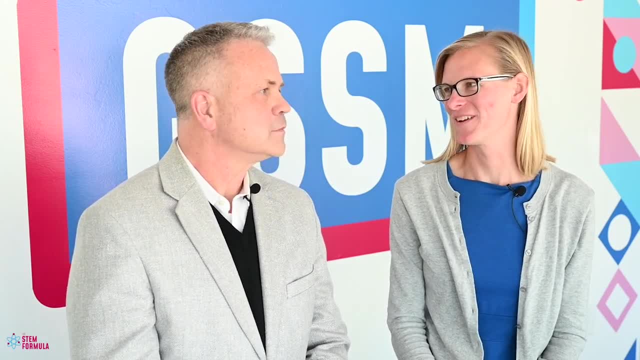 Uh, one thing that really stood out to me, Michael, was her emphasis of using real life examples and, uh, the small demos that she does throughout her class to to really bring home the fact that physics is something that's really important. 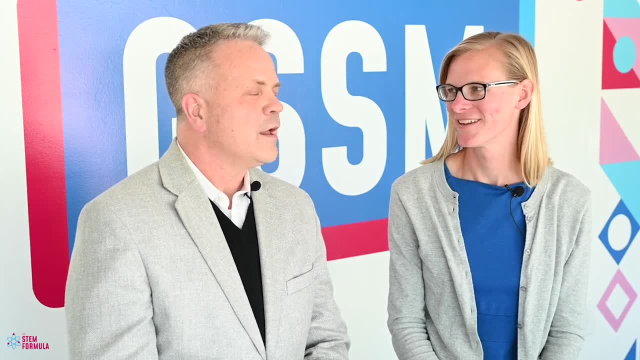 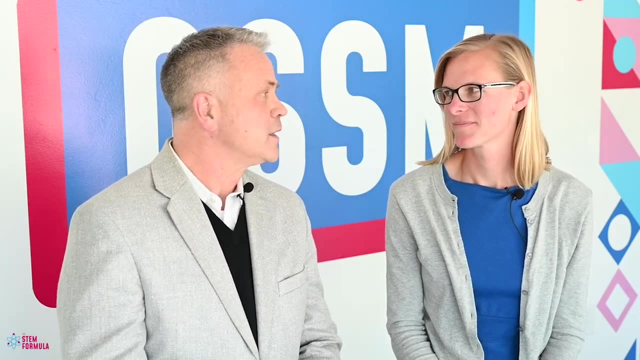 It's not something that you see in your everyday life. It's not something abstract. Yeah, I liked how she brought up teaching sports and and teaching music through physics And that was really interesting. Do you do anything like that in your math classes? 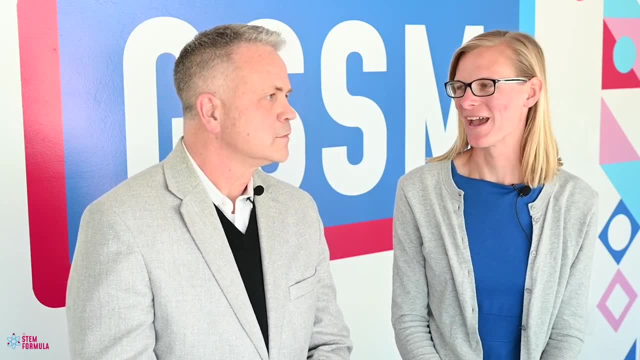 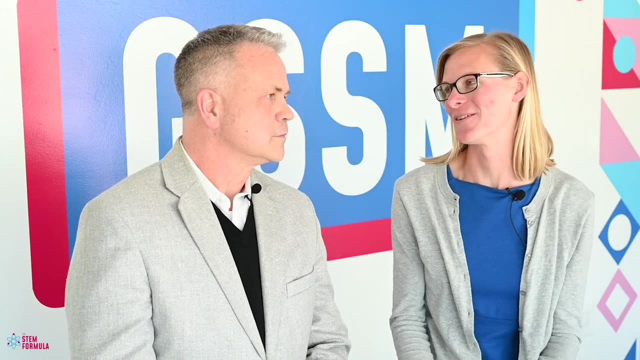 Yeah, And it depends especially on which math class that I'm teaching. Right now, though, I have a cryptography class that I'm teaching, where our whole emphasis is on cryptography and how- how math is used in that um, in our everyday life. 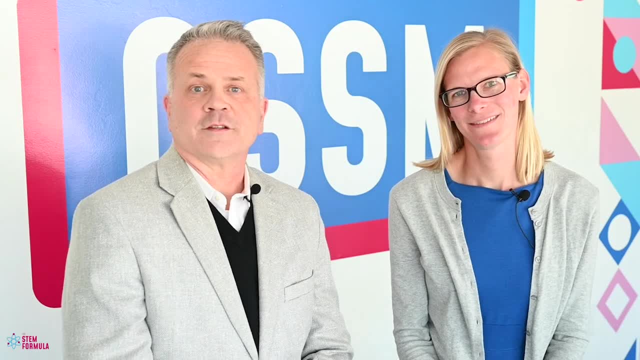 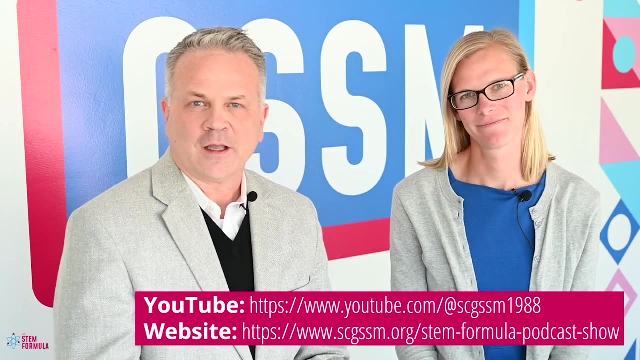 So, yeah, Well, we really appreciate you watching the show, and you can find all of our episodes on our YouTube channel. We're on the STEM Formula webpage. We'll put that information here on the screen. We'd also love to hear from you. 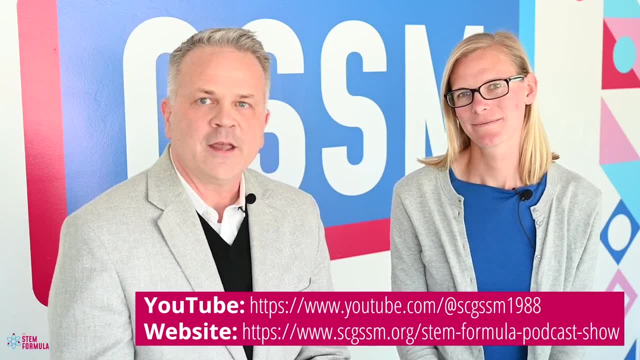 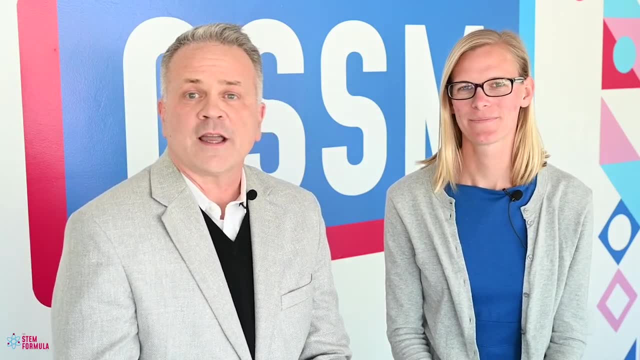 So you can just Google the South Carolina Governor's School for Science and Math and you can look for Michael Newsome Or Nicole Krager And send us an email. Let us know if there's anything that you would like us to do or give us some advice about the program. 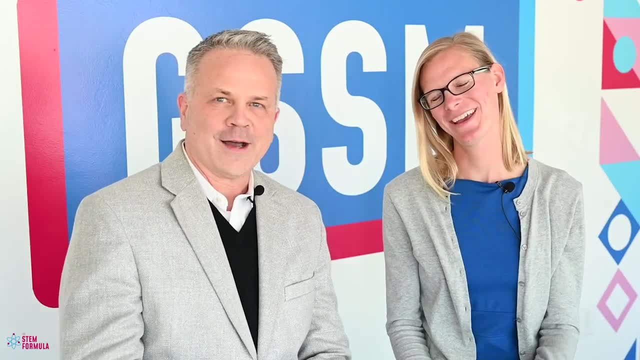 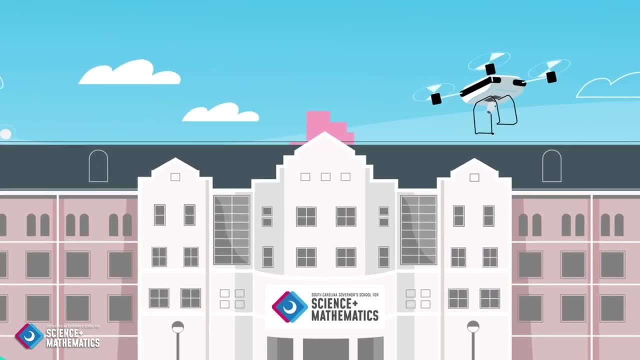 Well, until next time, Keep learning and growing Bye-bye. GSSM is South Carolina's nationally recognized STEM high school for academically gifted students. Take your education to the next level. GSSM residential and STEM foundations are for grades 11 through 12.. 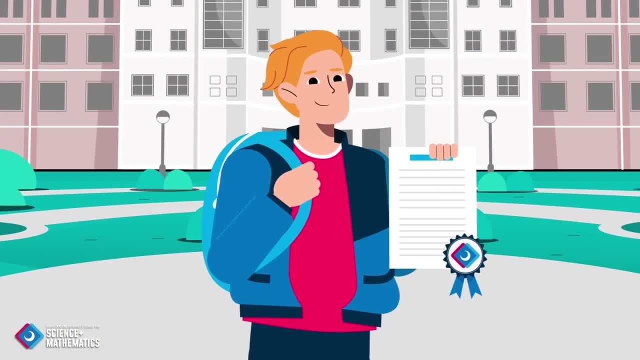 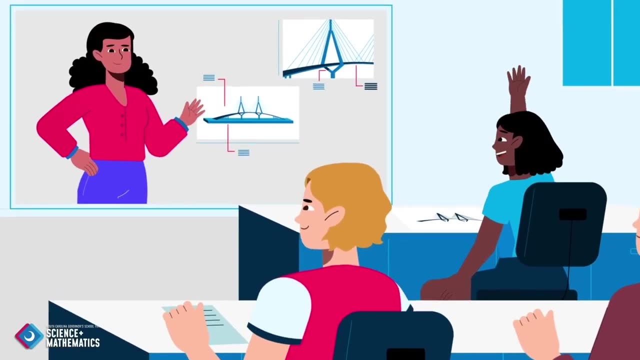 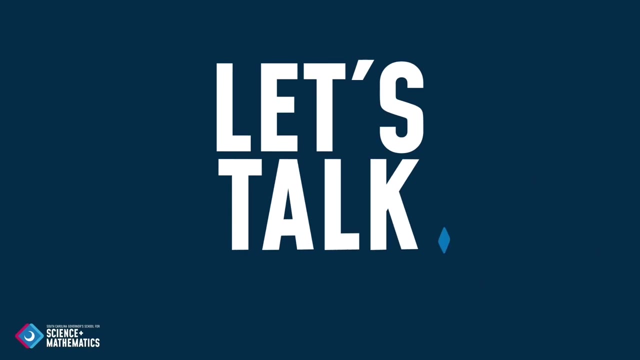 Summer research and international travel lead to earning the distinguished GSSM diploma. Accelerate is GSSM's engineering program for grades 10 through 12, taught virtually in real time at participating schools. Students can earn 50 dual enrollment credits. GSSM offers all these opportunities, tuition free. Let's talk. 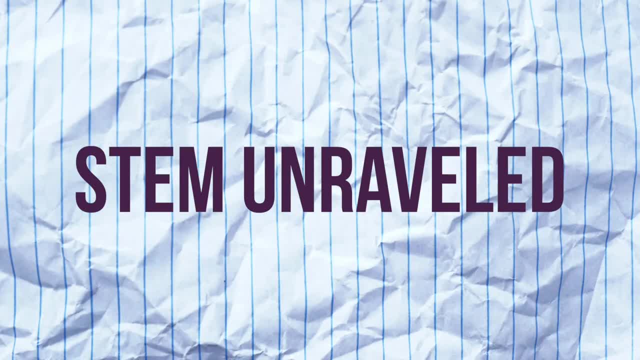 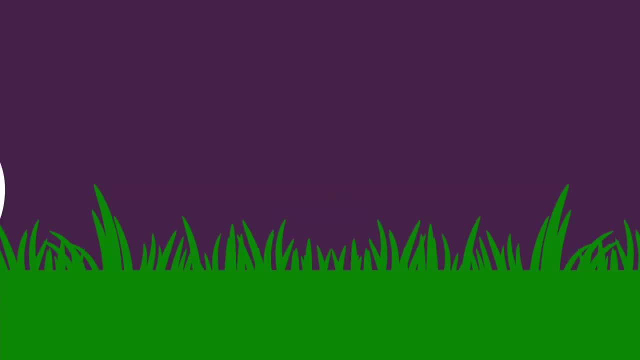 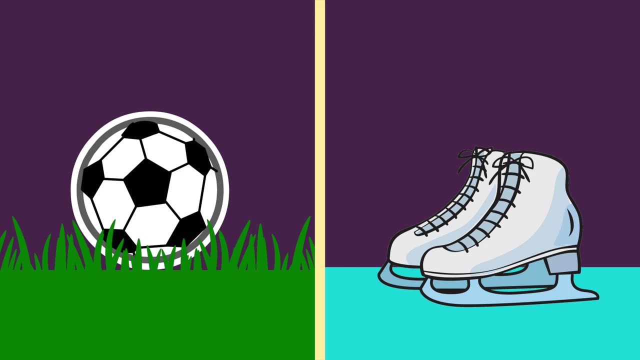 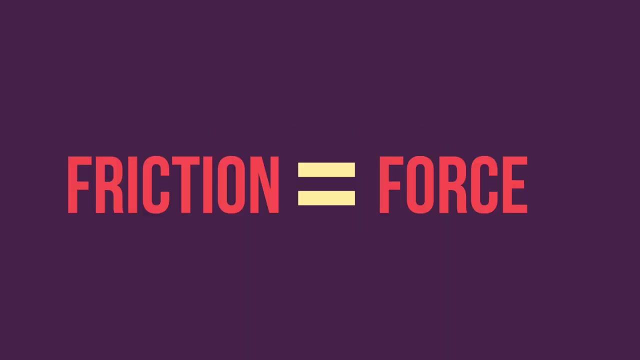 Have you ever wondered why a ball stops rolling Or why you use ice skates to move on ice? The answer is friction. But what exactly is friction? Friction is a force. It's measured as the amount of resistance that pushes against an